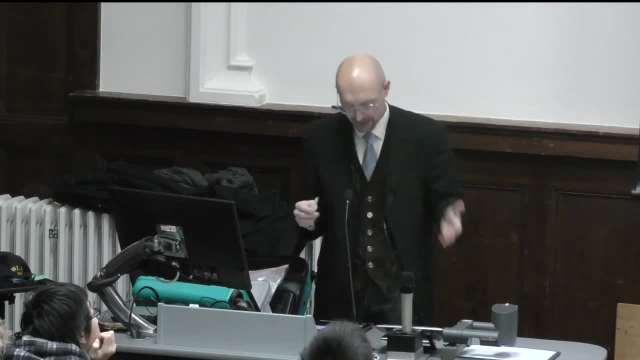 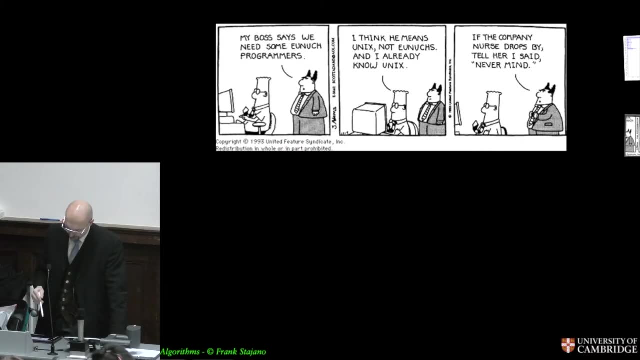 numbers. they could be characters, they could be bytes. If we think of bytes, then the bytes could represent anything. This is a digitized version of the picture that appeared in the newspaper, and this strip has been encoded in a bitmap file- Windows bitmap file that stores each pixel of the image as one. 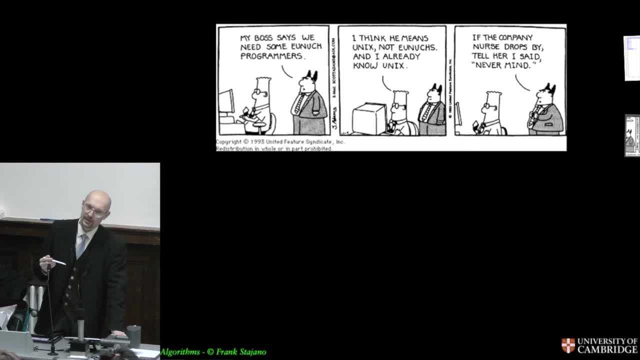 byte And the bitmap also stores a byte being an index, into a lookup table of 256 possible colors. Now, all the colors that are used in this case are between black and white and some grays, but the bitmap could also look at other colors which are not used in this case. 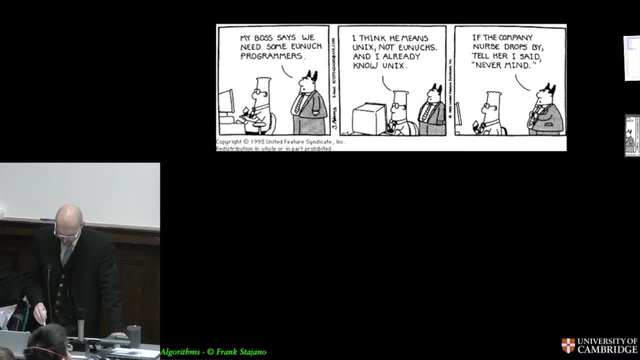 Anyway. so for each of the pixels in this image, the Windows bitmap file stores a byte and plus two pixels in this image. so a byte plus a number of pixels and then a number of pixels, some bytes at the beginning for some header information. so this is happens to. 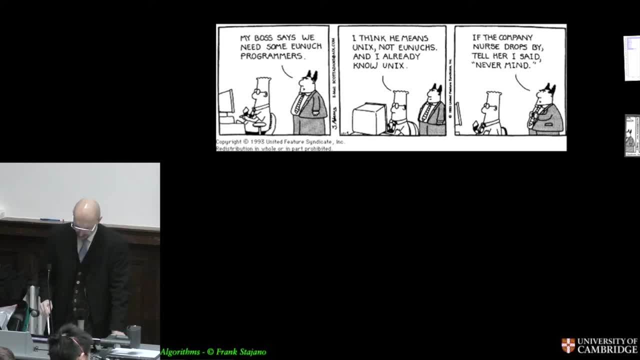 be 600 pixels across by 219 pixels down. so that gives us one, three, one four hundred pixels plus some junk for the header, another 88 bytes of header, and that's the total size on this. now, if I look what bytes are in use in here, I can run this through accounting. 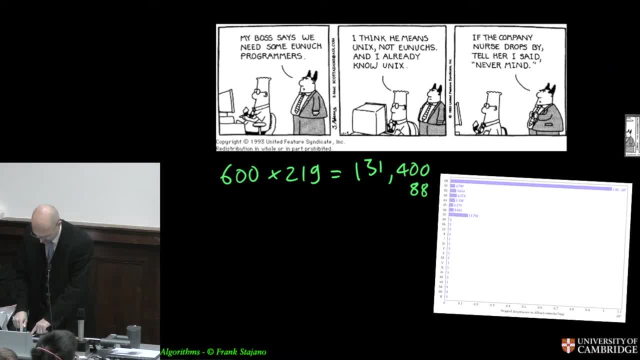 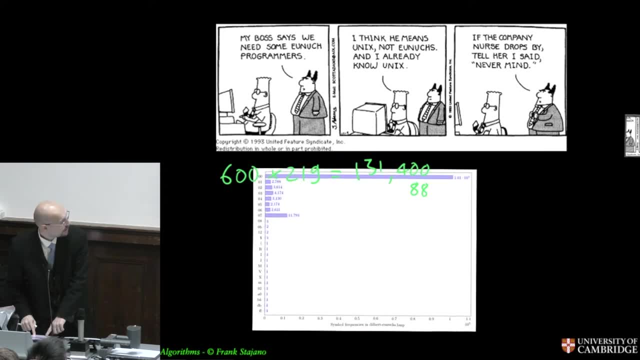 program, and I've written such accounting program. as you can guess, it's not difficult. it gives me a histogram like this, of how many times each byte is used. so on the left here I have bytes represented as either hex number or, if they're printable, the printable version. not that the printable version means anything in. 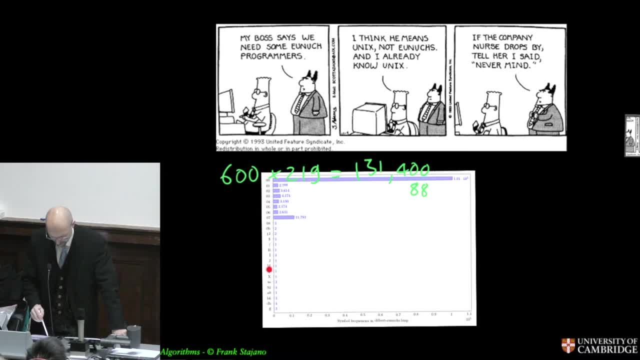 this case and matters. I should have just put the hex value for everything, but I had written the counting for another purpose, so I just recycled it. and this, this bar, says that the zero, zero byte is used basically a hundred thousand times. these other ones, one, two, three, four, are: 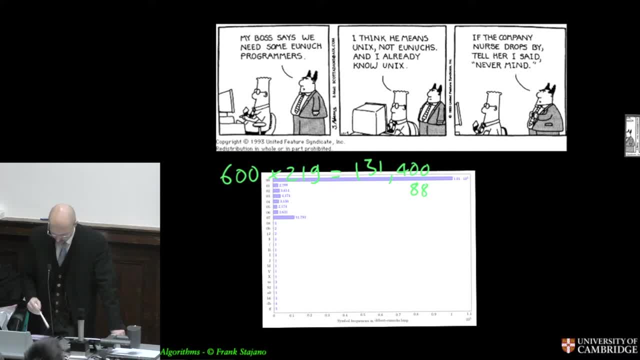 used a few thousand times each. this seven is used 11,000 times, and then these other ones. there's a tale of things that are used just a single digit number of times, three times, two times, two times. so it's an easy guess that this is the. 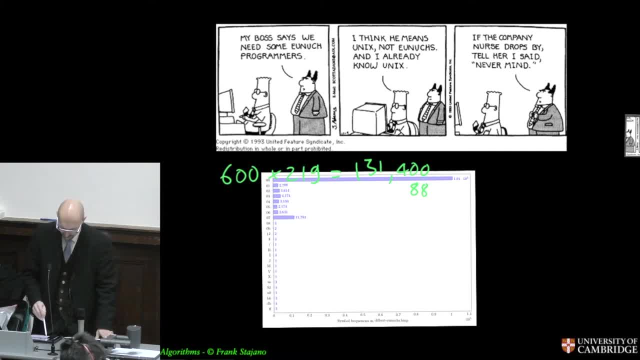 the white, this is the black, these are some of the grays that are in here, and these are some some grays that rarely occur. you could imagine just getting rid of these and the picture wouldn't noticeably change. if you had just this and this, it would still be recognizable. 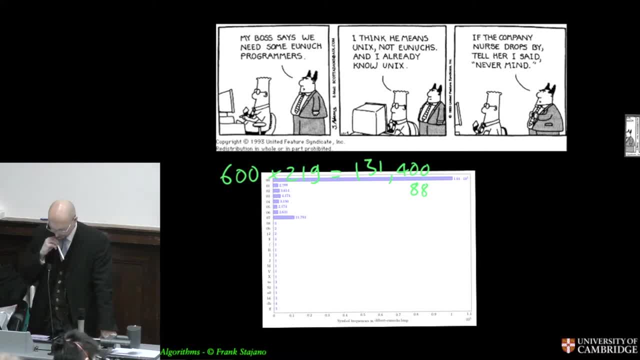 we would just look a bit more crude in the details, and an obvious way to compress this would be just to get rid of these, and I'm left with only seven- no, actually eight- different values to encode, which don't really need one byte each. eight of these will only need three bits each, and so I already get a. 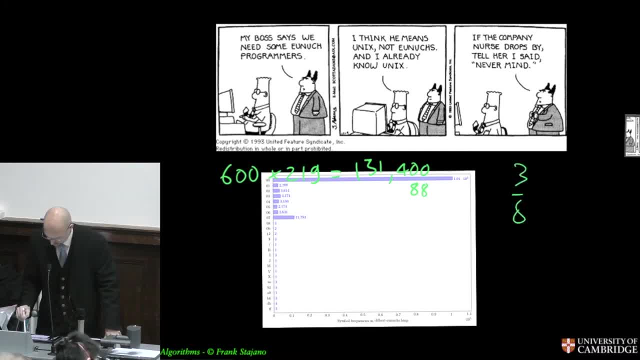 reduction by a factor three, eights, in this number of bits that I need to store in order to encode that and that's nothing special. but I'm just saying I don't want to pretend that I am getting a big gain when an obvious big gain could be had with a small number of bits. but I'm just saying I don't want to pretend that I am getting a big gain when an obvious big gain could be had with a 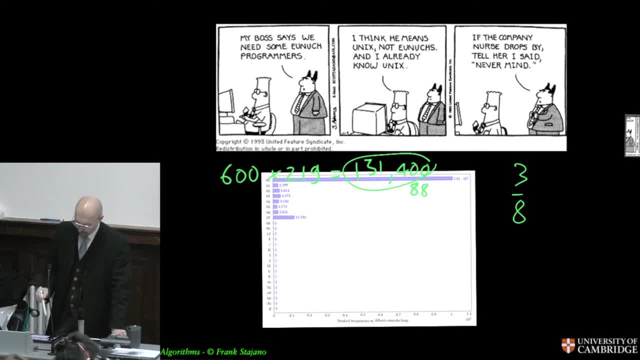 much simpler techniques. so, but still, compared to the value this number times this number, is there a more efficient way of encoding this picture based on the same idea of Morse code that, if there is something that I know about the frequency of occurrence of the various symbols in my input stream, if some 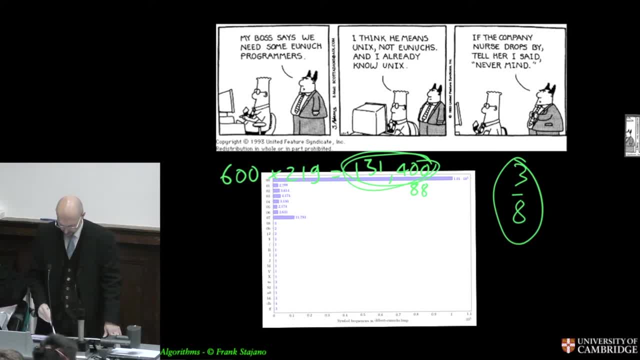 symbols occur much more frequently than others. this one occurs a hundred thousand times and these other ones a few thousand. this one ten thousand. then it might be a good idea to make the symbol that occurs a hundred thousand times shorter than these other ones, and then, even if some 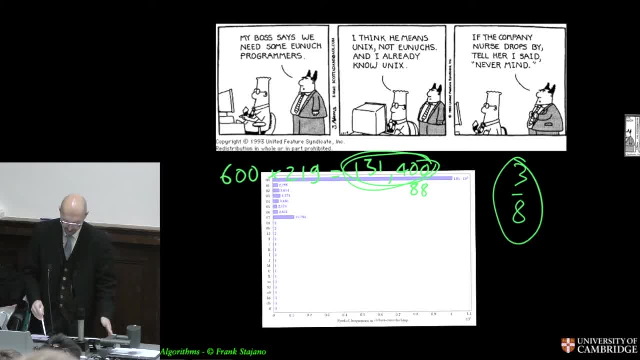 of these become longer because on on average, they will all be three bits. if I make this one shorter than three bits, some something will have to be four bits, but if it occurs so much less frequently, I may still have the gain overall. so the idea of the family of codes that we are 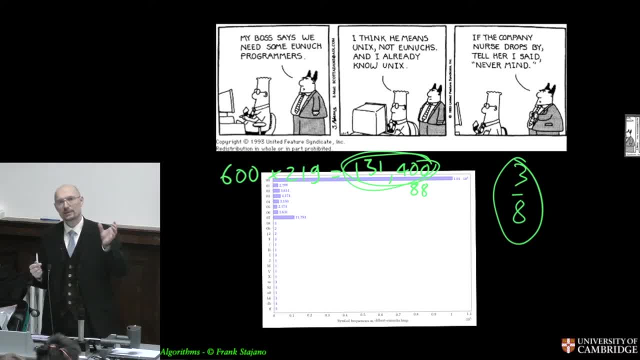 looking at is to take symbols that are encoded with a fixed number of bits each and make a bijection between those symbols and other code words, which may have variable length in bits, and allocating shorter codes to the more frequent source symbols, so that these shorter code words will give some saving. 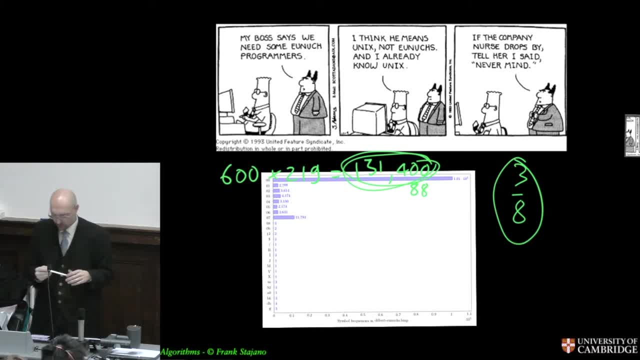 when they are strung together, and this is something that you can only do if you know something that you can only do if you know something that you can only do, something that you can only do if you know something that you can only do if you know something about the frequencies in the input. if you don't, 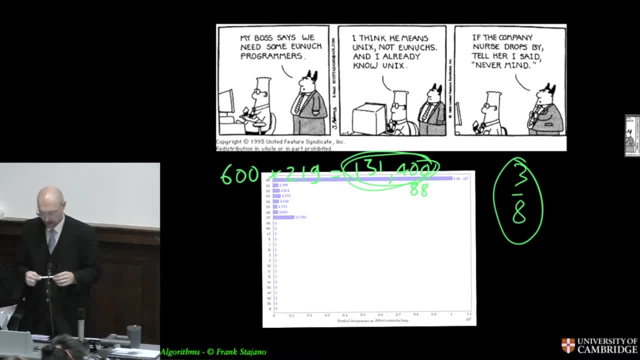 know anything, then there's no reason to make any symbol any shorter than any other and in fact it is possible by this technique to make the output longer than the input, which is not advantageous for the purpose of compression. but if you, if you know about the implicit, is going to use them properly, then it is possible to 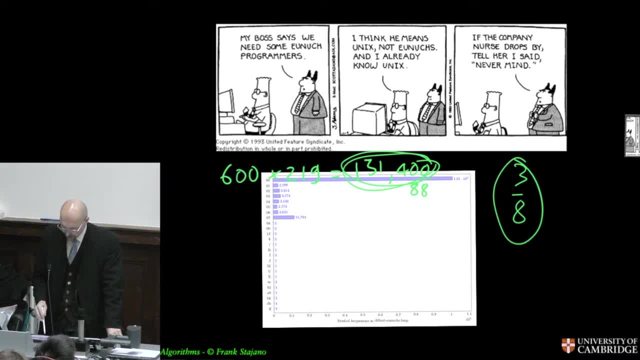 make a gain if I'm going to encode things into mean one, followed by two ones, followed by a one, followed by three ones, or if he was just individual ones, or if you do this one long code, we did multiply them. if you code of five ones plus another one of five ones, 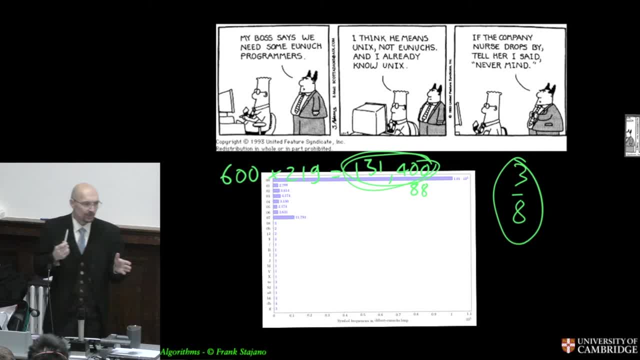 How do I know? So Morse code cheats, because Morse code adds extra space between the dots and dashes. We are not allowed to do that. We only have zeros and ones. So if we are not allowed to cheat in the way Morse code does, what we need to do? 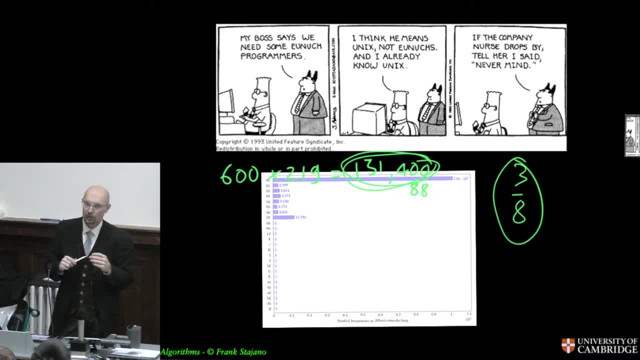 well, one solution to that issue is to make a code where it is uniquely determined which code word can come out of a string, no matter how long it is, because no two code words start in the same way, So no code word is a prefix of any other valid code word. 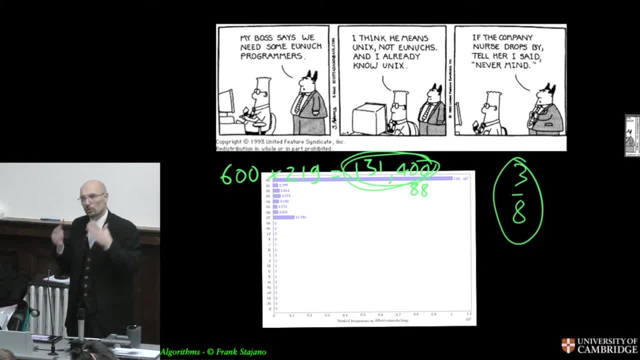 Are you with me? So not all possible choices of code words enjoy this property, but it is possible to decide. this is gonna be one of my rules. I'm gonna only make codes where the family of code words never has one code word as a prefix of any other code word. 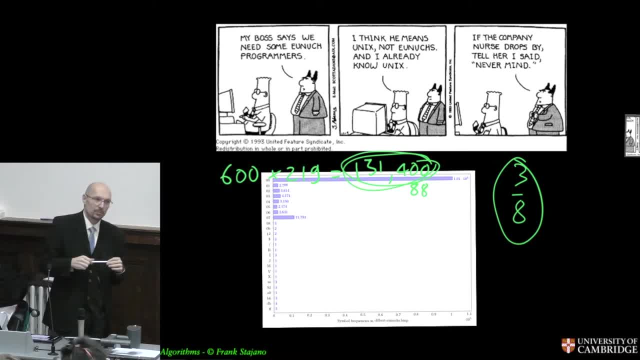 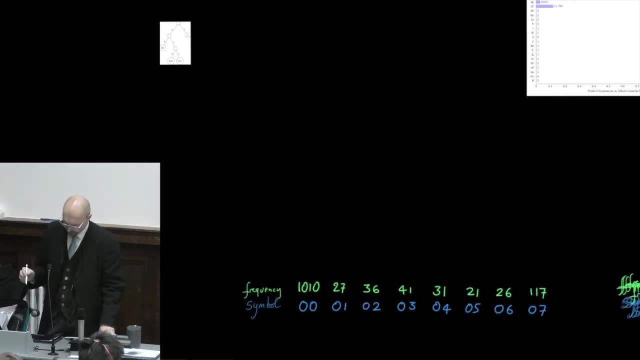 This family of codes is called prefix codes. If we were logical about it, we would call them prefix-free codes, but the custom is to call them prefix codes. How do you build a prefix code? If you think about it, a prefix code is what you get. 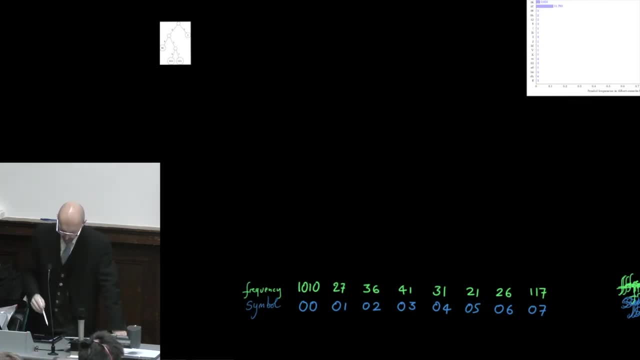 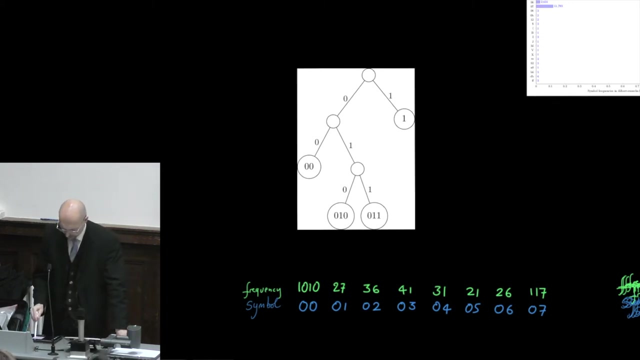 when you have a tree like this one, where every node is either the parent of two children or the parent of no children. So this node is a parent of two children, this parent of two children. this one is the parent of no children. There's no node that is a parent of just one child. 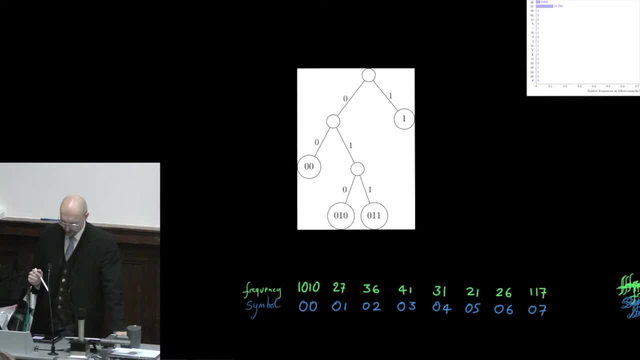 In this type of tree. you can call the nodes that have no children, the leaves of the tree. The leaf of each tree is associated with the code that's obtained by taking the bits on the branches that lead to it from the root. You call left, zero and right one. 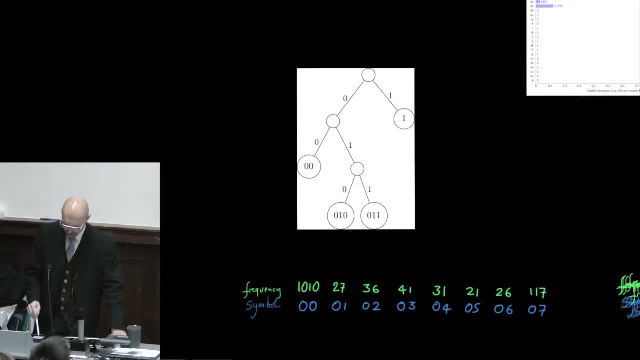 Then, from the root, you take the zero child and the one child. zero child and one child, zero child and one child. So the code for this is zero zero. the code for this is zero one zero code for this is zero one one. 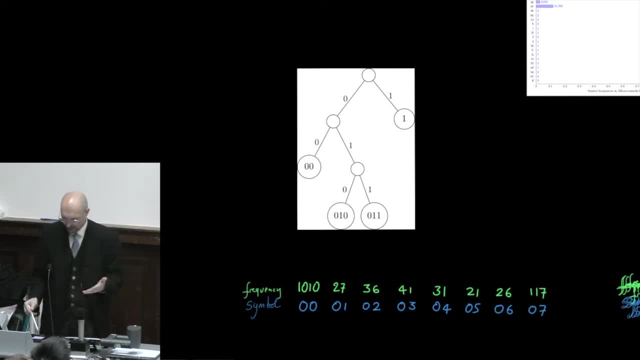 and so on. And it's fairly obvious from this example that if you build your code in this way, it is impossible for any code word to be a prefix of another code word, because for a code word to be a prefix of another code word, you would have to have a code word somewhere and then continue. 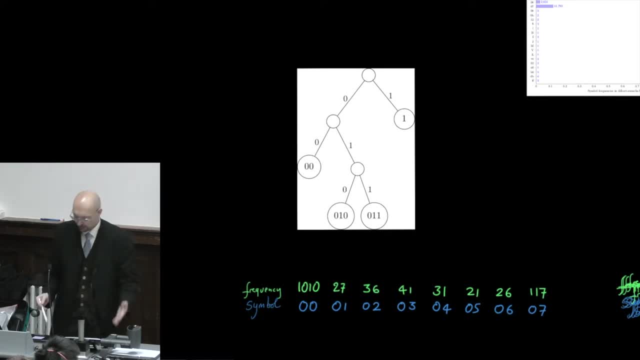 with something else after it. But you can't do that if you said that you can only have nodes that either have no children- in which case they are leaves, and that's where the code words live- or they have two children, Because if you are a code word, then you're not going to have. 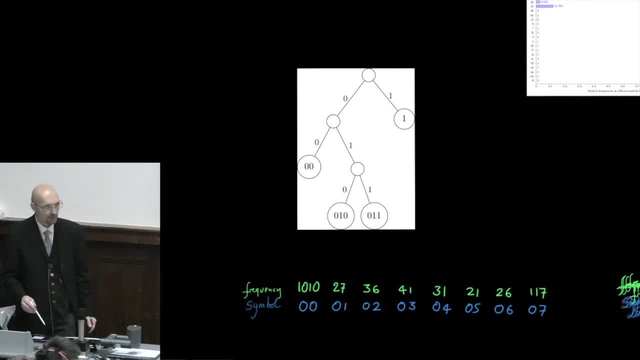 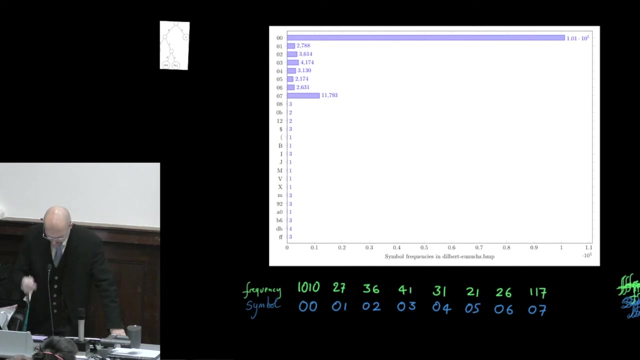 children, you're not going to be able to continue to something else of which you would be the prefix. So this is a procedure for building a prefix code: Just build yourself a tree like that. So if we think of our frequencies here, when I was writing the handout, I was attempting to be pedantic about the distinction between: 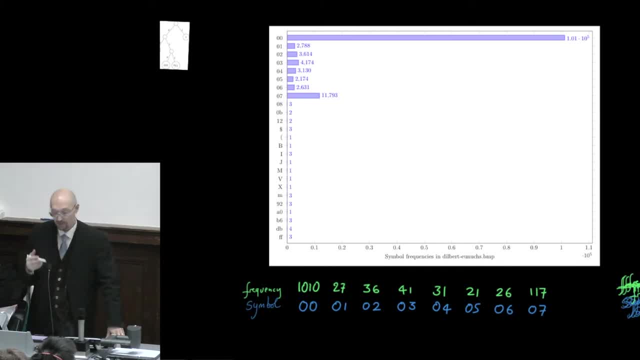 number of occurrences and frequencies. Some people might describe the frequency as more like the probability, so like the frequency of this one is one tenth of the total. So all the frequencies would adapt to one. but not everybody is consistent about this, So some people just say: 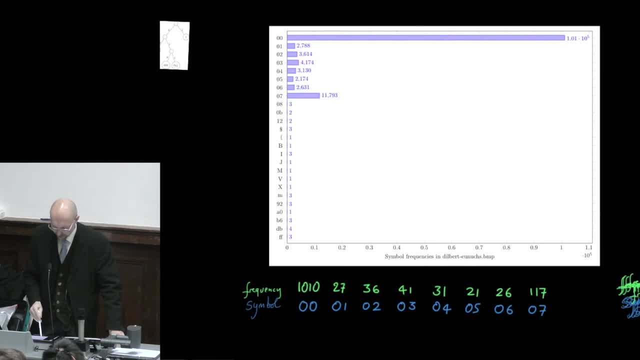 let's just put it like that, And I think also your book just says that if this occurs 2,788 times, then its frequency is 2,788 in the context of that file. So in that case you just take the total of all these and divide this thing by that number. 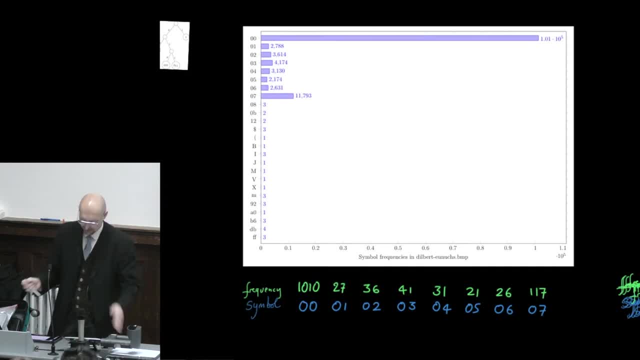 in order to obtain the probabilities or the things that would then adapt to one altogether. So for the purpose of not having numbers with too many digits, which would slow down the calculations, I've taken the numbers in here and I've just taken how many I've truncated. 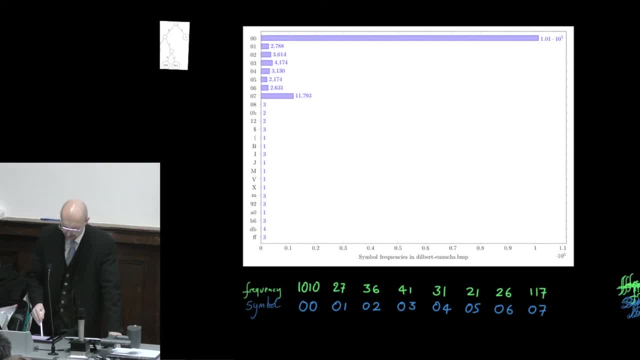 it to the hundreds. So if this is 2,788, I call it 27.. 3,614, I call it 36. And I copy them down in here. So the symbol 00 is worth 1,010.. 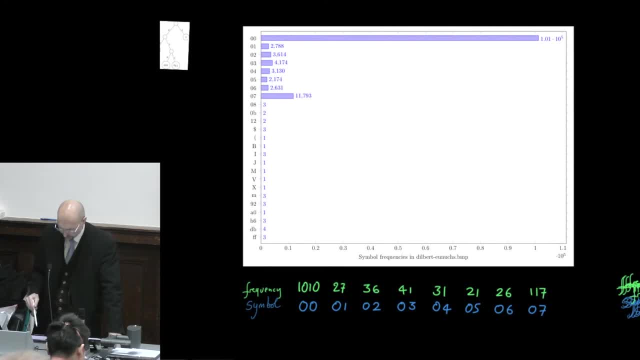 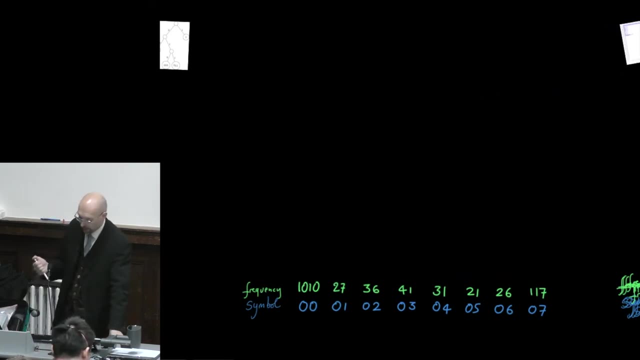 The symbol 01 is worth 27.. The symbol 02 is worth 36 and so on. So I can- this is a representation of this histogram- So I can make any code I like within prefix-free codes, just by building a tree out of these. 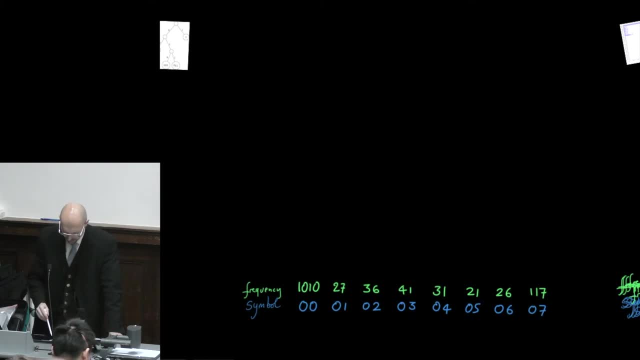 leaves. So I build a tree bottom up And what I would do is something like this: I take two of these and I make a node. I take two of these and I make a node. I take two of these and I make a node I don't have. 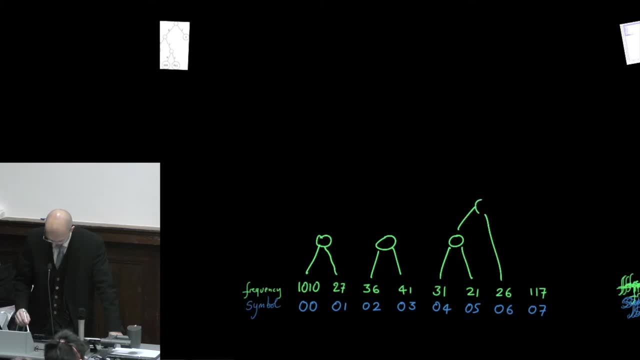 to. I could take this and this and I make a node. I could take this and this and make a node this and this. why not this and this? that's a tree, And so that would give the following codes. So this one. 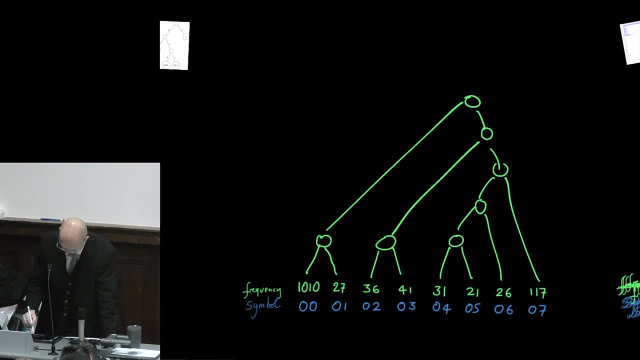 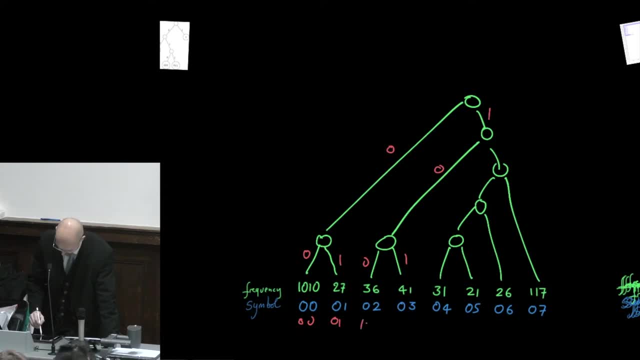 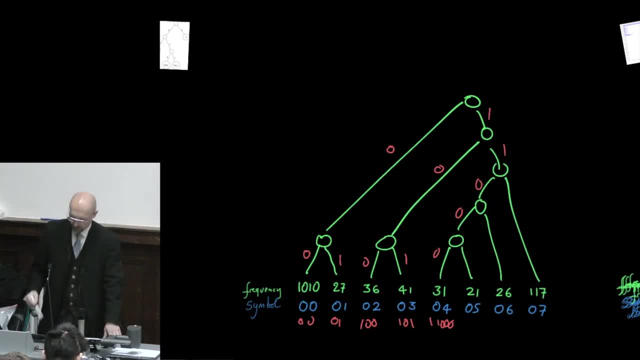 And I assign a unique code to each seemble in a way that ensures no codeword is a prefix of any other codeword. And if I did that I would have a code and I could it encode the original file in this. 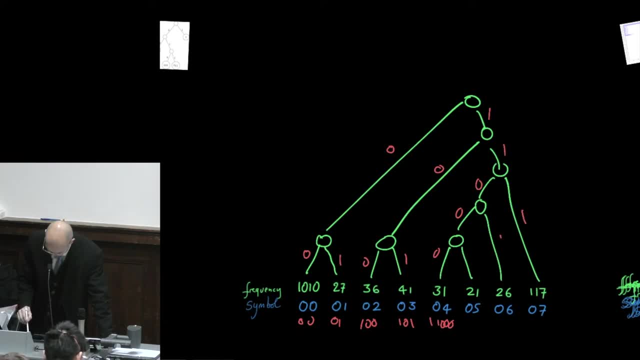 way, and I might ask myself How many? with one, one, zero, zero, one, one, one, zero, one, one, one one. I might ask myself how much? how many bits would I use if I use this code instead of the original code? you have a question? yes, oh, excuse me, I'm very sorry. yes, if I do this thing, which? 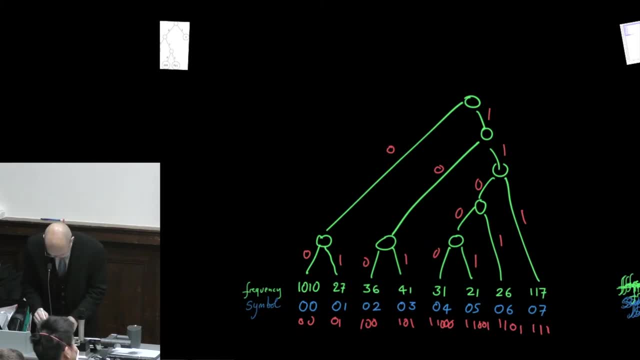 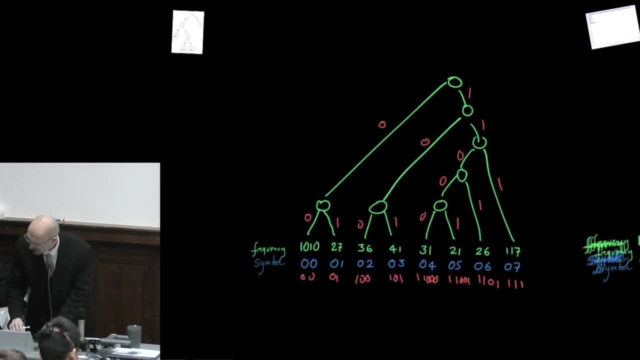 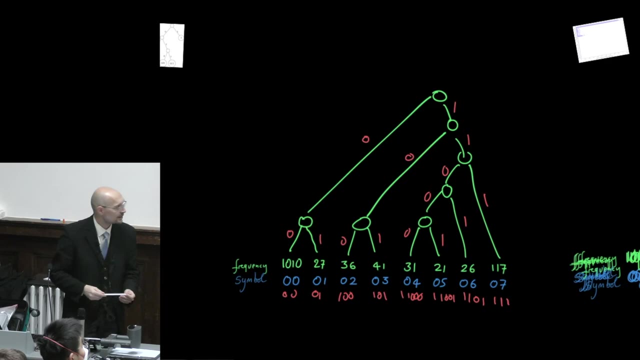 is because they still haven't fixed the projector. it's not projecting as much as my screen. then please feel free to actually make sounds and say: hey, I am not seeing what you're doing, we are wasting time, you have to restart again. so don't be so polite that only if I look in your direction I would notice. if 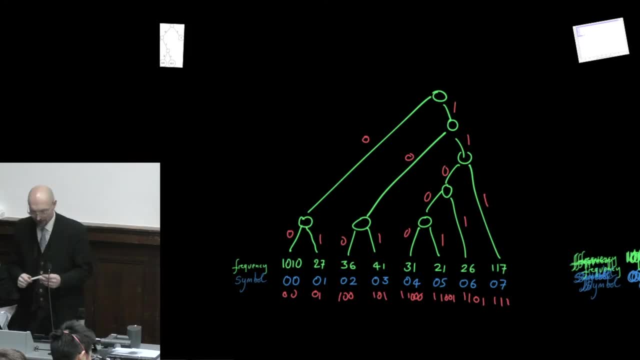 you don't take ten minutes for me to look in your directions. we are stuck, so my apologies for this. I was drawing at the bottom of the screen the I code words that you obtained by following through the branches and I hope I haven't made mistakes in copying and dumping. I hope one of you will alert. 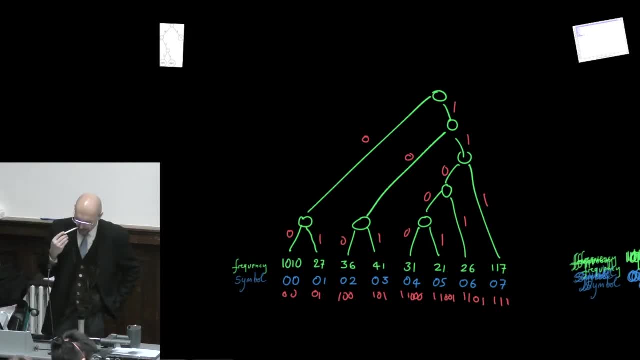 me if I have. so my next job is to say how much would this cost. so the cost of a code, I can. I can in terms of the compression. I can just talk of the cost of a code in general, regardless of the input, if I know the frequencies of the. 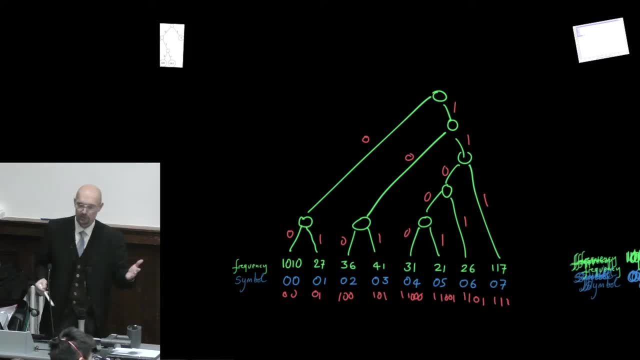 input, input symbols. then if I have another input with the same frequencies, that's fine. if I have a much longer file, so long as it has the same frequencies, the efficiency of the code on it will be the same. so I can talk about the cost of a. 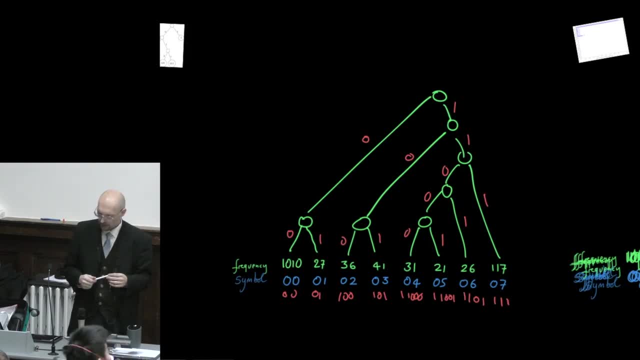 code as basically the average length of the encoded symbol through that code, weighed by the frequency of the symbols. am I making sense? so if I have the source where every source symbol is encoded with the same number of bits- in my example 8 originally or 3- if I get rid of the total wastage, then clearly, 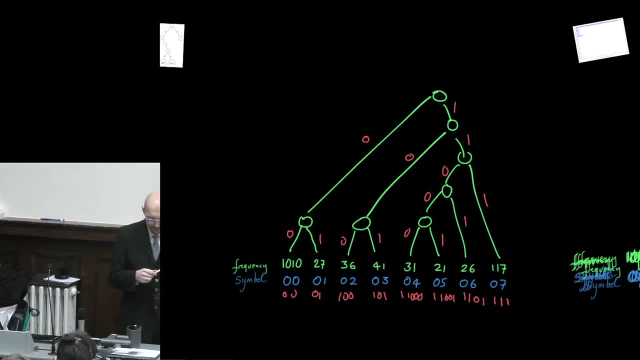 the average of space used by each symbol is 3 bits, because it's the same for all of them. but if I have a variable length code like this one, some bits are encoded, some symbols are encoded with 2 bits, some symbols with 3 bits, some symbols with 5 bits, some symbols with 4 bits. on average, what's the? 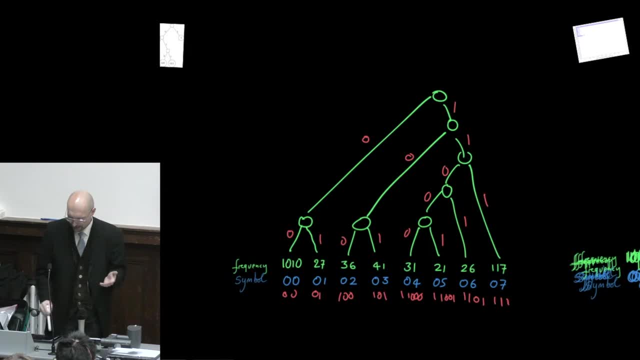 average length? well, it's not the sum of these things divided by 8. it's the sum of this weighed by their frequencies then, which should all be divided by the sum of the frequency, so it adapts to 1, and then then that's the average length of the symbol. so, if I have a variable length code, 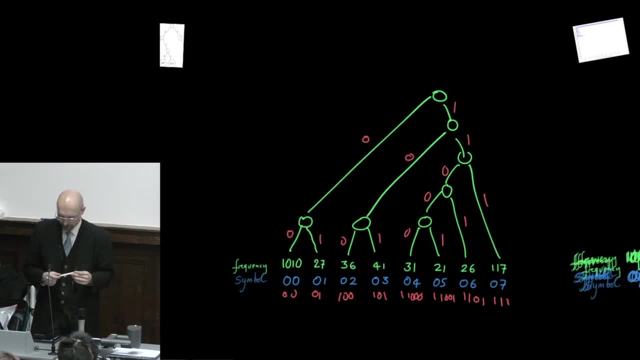 that will give me the weighed average of the length of these, and if this weighed average is less than 3 bits, then I'm using less than 3 bits per code word and I am making a compression. and if it's greater than 3 bits, then I'm not making. 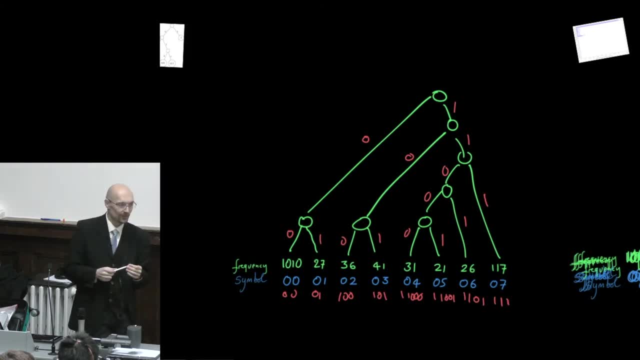 compression, and it's not a good code to use if I wanted to compress. am I making sense? so the sum of these frequencies over here- okay, then, and plus I'm- I'm adding up all these things here- and 10 plus 27 plus 36 plus 41 plus 31 plus 21 plus 26 plus 1 1, 7, is 1309. 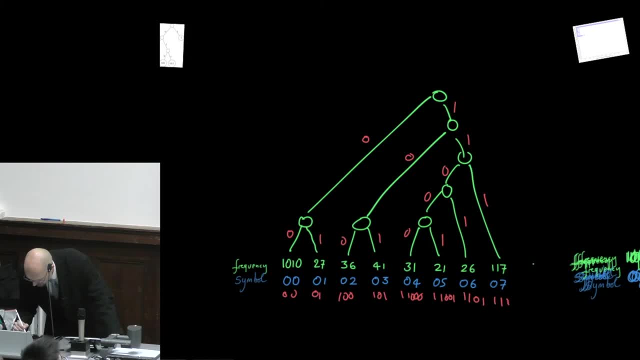 so the probability of each of the inputs symbols would be the number that I have here divided by 1300, 1309. and if I multiplied that fraction by the length of this and added them all up, so, and then divided by thirty or nine, plus times two bits, this one divided by this, times two bits this one divided by this. 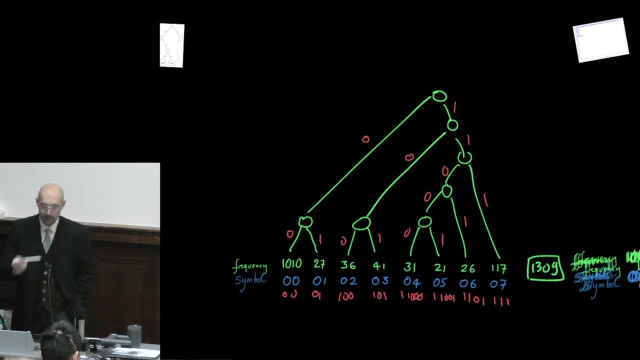 times three bits and I added all these up, that would be the cost of my code. Every time I decide to pair up two of these, I am making a choice And you can see. if you're smart, you will have noticed the isomorphism between. 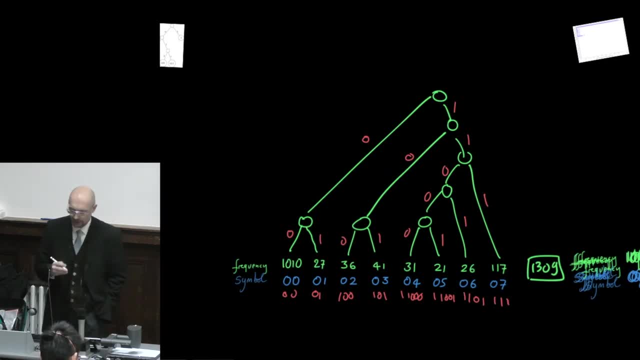 this and a problem. we did a lecture or two ago where I was trying to multiply matrices, where, ultimately, the choices I was making was which two matrices do I multiply at a time, And so this gave rise to a number of possible trees that I could rearrange this into. 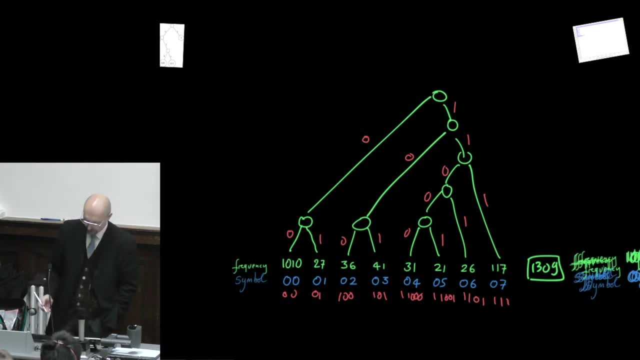 And there were a Catalan number of trees which grows more than polynomially, And so I said I don't want to look at all these trees. And here is the same. There's an exponential number of these trees that I could build. 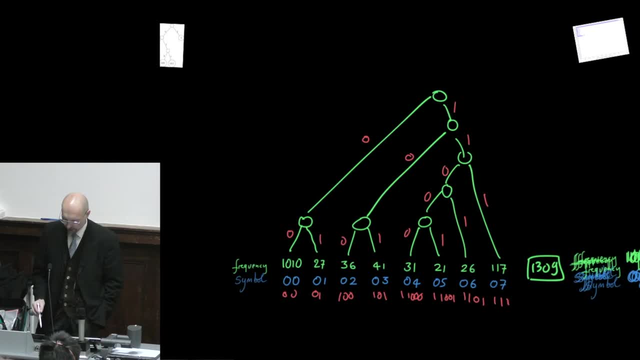 And I don't want to have to look at all of them, But each time that I pair up two things, I'm making a choice, And I would like to make the greedy choice. I'm talking of Huffman codes as an example of greedy. 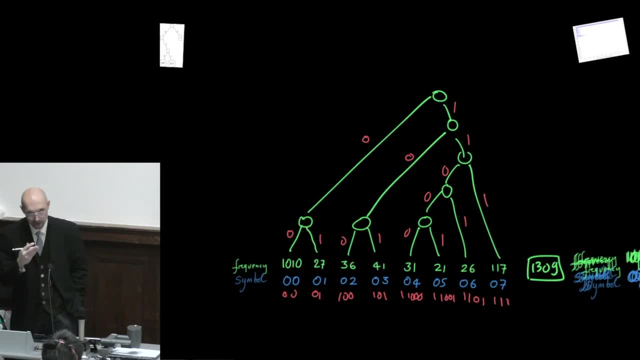 Where is the greed in that? How am I making a greedy choice? Well, the greedy choice would be the one that leads to the least expensive code, And so, if I could somehow define what is the contribution of each of these decisions to the final cost of the code. 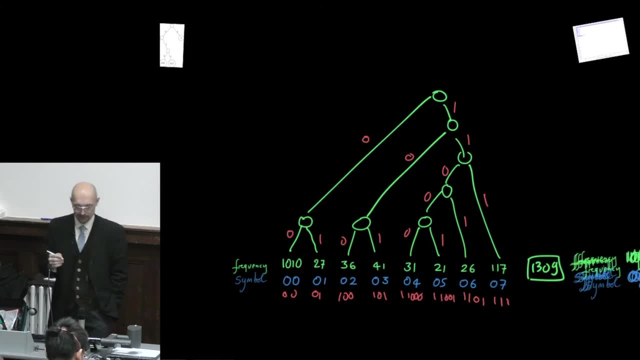 then I could take the decision that costs the least. So pay attention to this, Otherwise you will get really lost in what I do next. And when I was rereading my handout to prepare today's lecture, that's the point where I said I must explain this really clearly. 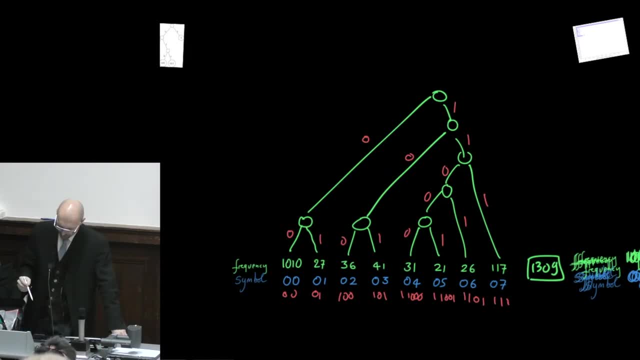 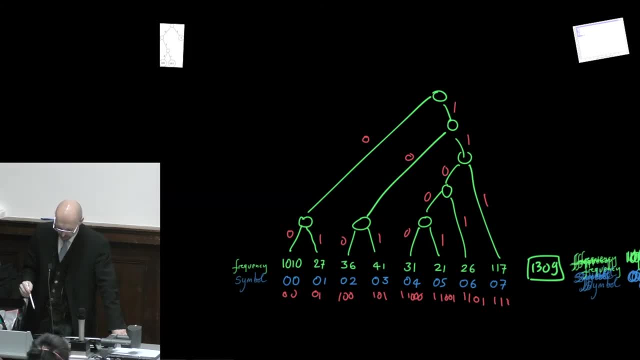 So, So, So So. The total cost of this code is given, as I said now several times, by the length of each code word weighed by the frequency. So the length of each code word is the length of the path from root to leaves. 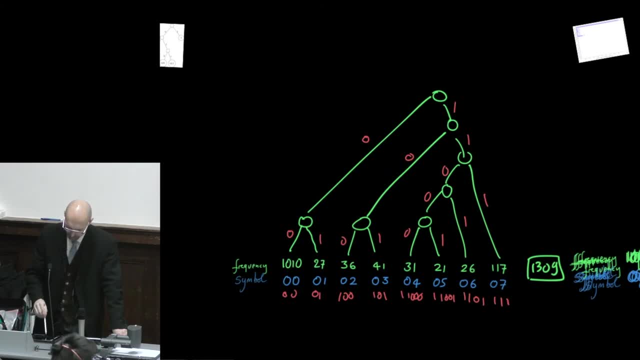 So I can say the cost here is this length two times this, This length two times, and I'm ignoring the division by 13, and I can do that at the end, So when I'm still in the process of building up this code, 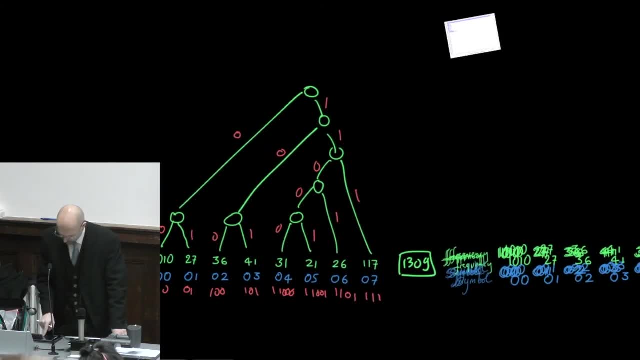 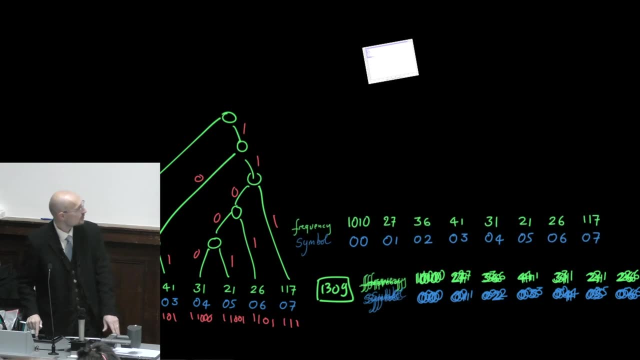 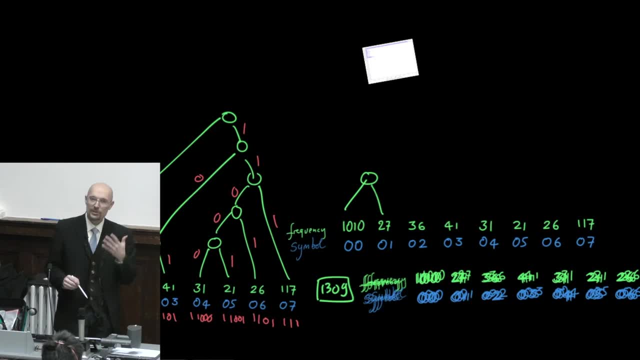 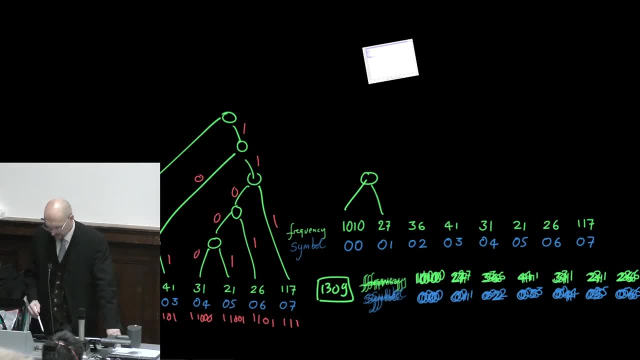 It's not a code because it can't encode anything. It can't encode the arbitrary inputs with the symbols, But what could I define as the cost contribution of this towards the total cost? Well, one definition that I came up with which I think is sensible and consistent: 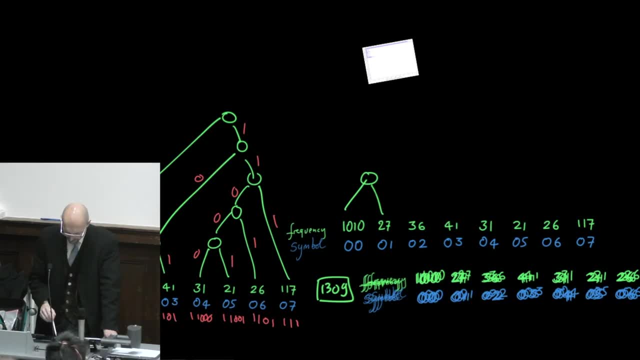 with the rest of the stuff I said is let's take the length of each code word. So at the moment I've only made code words for this one, which would be zero, and this one, which would be one, And these ones don't have a code word. 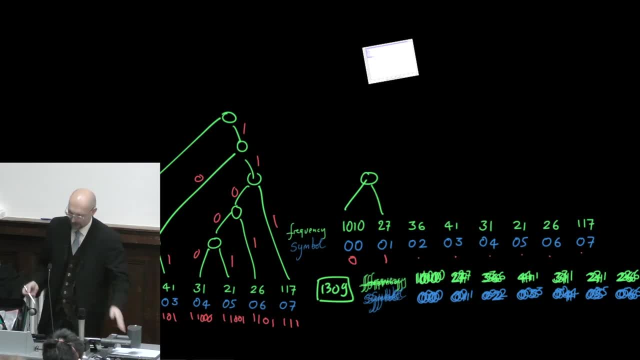 Because they don't have a code word. code is incomplete and doesn't work. But because they don't have a code word, the length of the code word is zero And so they don't cost anything. So, although this code is incomplete, 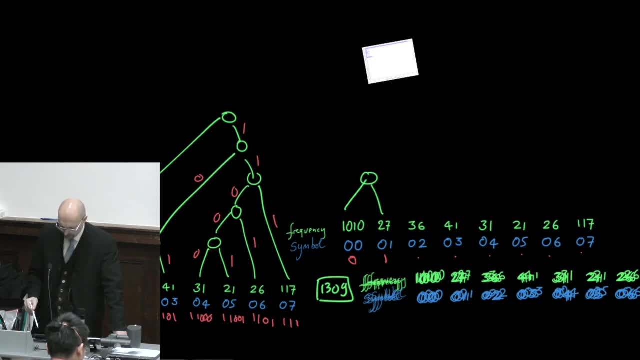 its cost would be one for this and one for that, So the cost would be one times 10.10, plus one times 27.. So it means I just add this up, so that's 10.37.. And I write this cost in here. 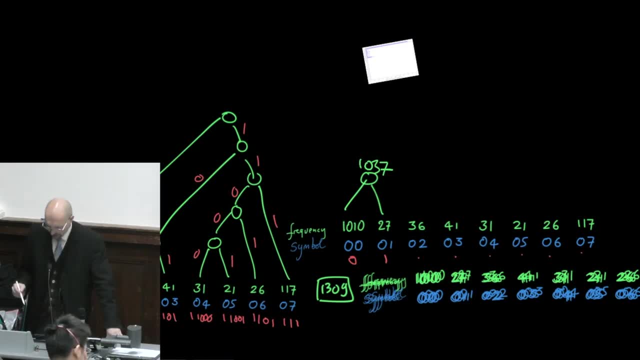 If I were to take another decision, which might be, I'm gonna take this one and this one. What would be the cost of the code resulting from all that? Well, the new code would now have this, and it would also have a zero for this and a one for this. 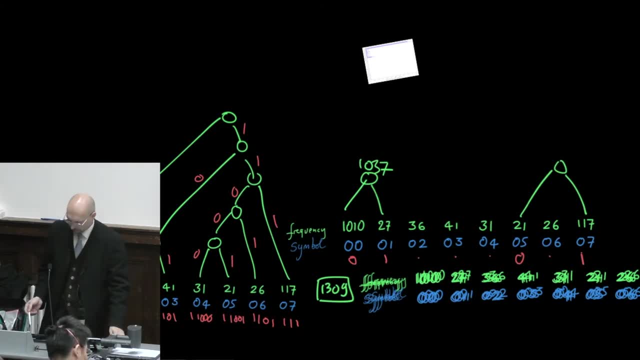 We can see it's not a proper code because there are two symbols that reuse the same code word and two other symbols that reuse the same code word. So things are still incomplete. it's not properly a code, But on the way to making another code. 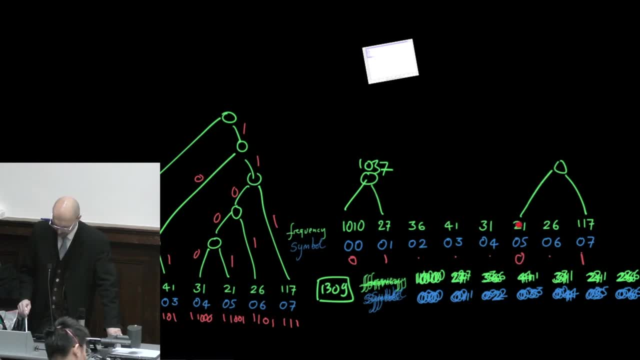 I have made another word of length, one which is gonna be used 21 times, and another one of length one that's gonna be used 117 times. So the cost contribution of this new decision I've taken is going to be 21 plus 117,. 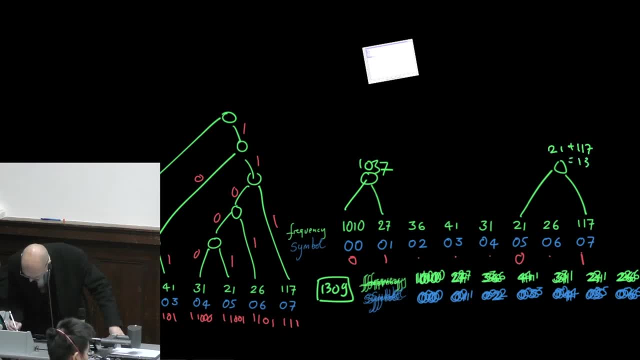 which leads me to 139.. So if I were now to add another node that doesn't take two leaves, but takes an existing node and a leaf, or an existing node and another existing node, for example this, what would I be making? 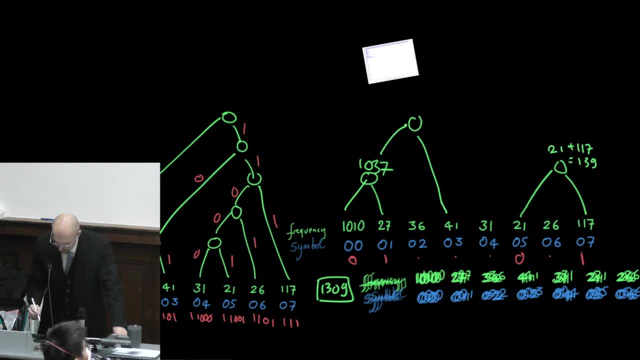 Well, I would be making a new code that's 00 for this. So this changes to 00,, this changes to 01,. sorry, Yeah, 01, this one changes to one, And so the cost of this symbol in the current code. 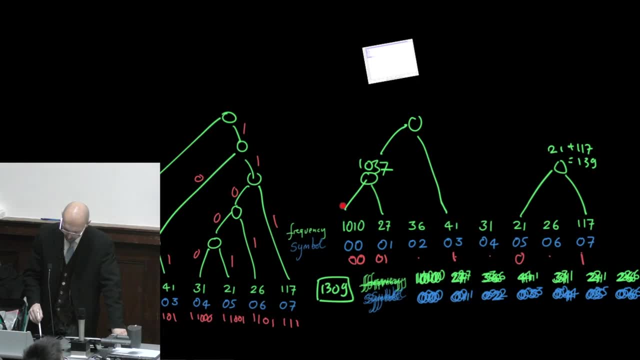 form so far, would be two times 1010.. The cost of this symbol would be two times 27.. The cost of this one would be one times 41. This one one times their own frequencies. But important, what is the cost of this particular decision? 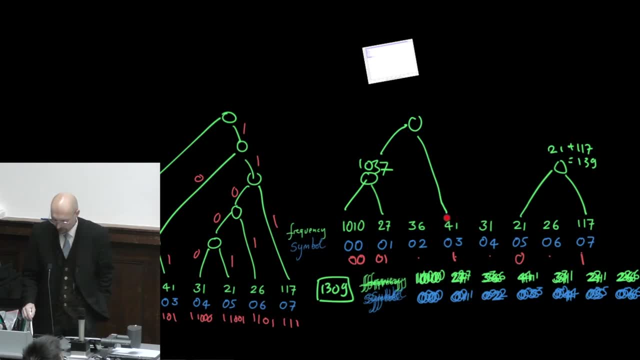 of merging this and this. The cost of this particular decision is the sum of all the things I just said, Minus the sum of all the things that existed before I took this decision. So the cost of this particular decision is just the increment in cost from the previous incomplete code. 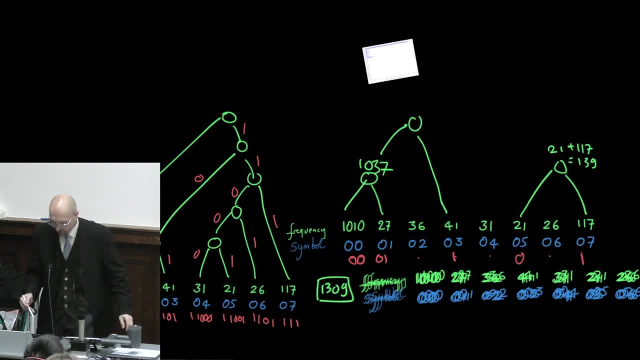 to the current incomplete code, And this extra cost is just adding one more leg to these two and one more leg to this one. That's a crucial point. Does this make sense? You can develop the algebra and see that this one is one. 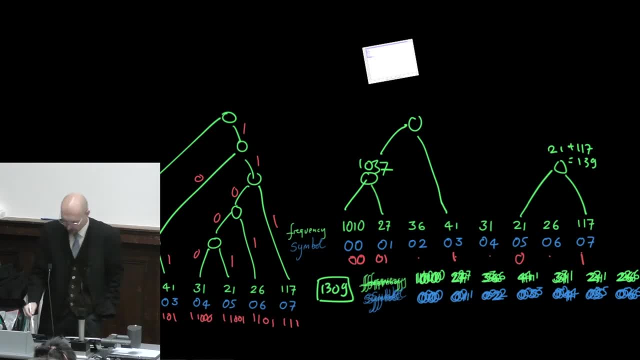 You can develop the algebra and see that this one is one, This one now becomes two, but you can subtract the one that you had before. So all that really matters is that each one of these extra things I do, each one of these, 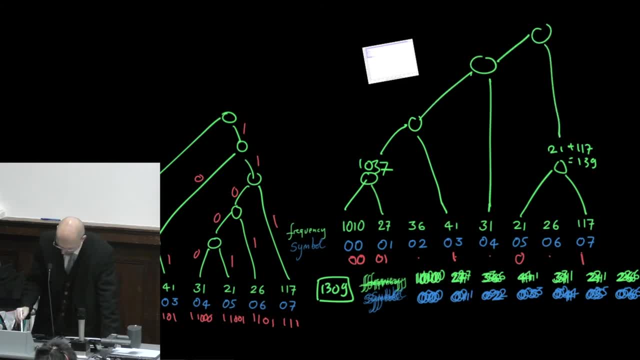 like that, just contributes its two branches, So one for this and one for this, one for this, for all of these, and one for this for these Right. So the contribution of this is actually, this times, the sum of all these three. 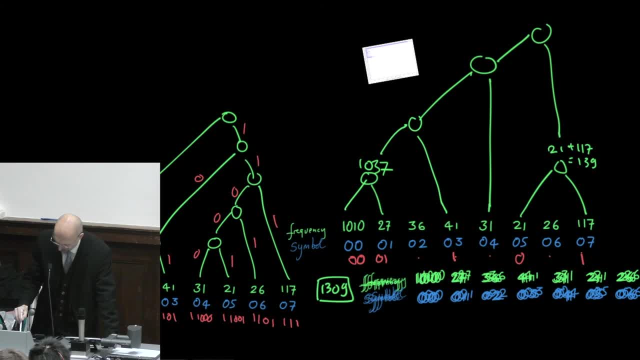 this, this, this, this, Not this one, because it's not part of this tree, And this one is the sum of this and this, But, cleverly, the sum of this- and this is already written in this node- And the sum of this, this, this, this, this. 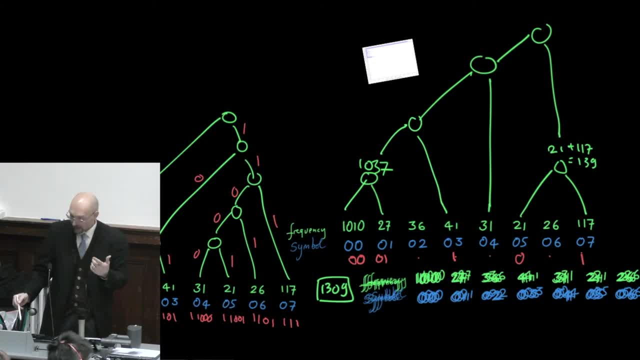 is already written in this node, because that's how I'm building them up. So really in each node what should go is the sum of the two nodes, that it merges Right. So if you were paying attention along, it makes sense. 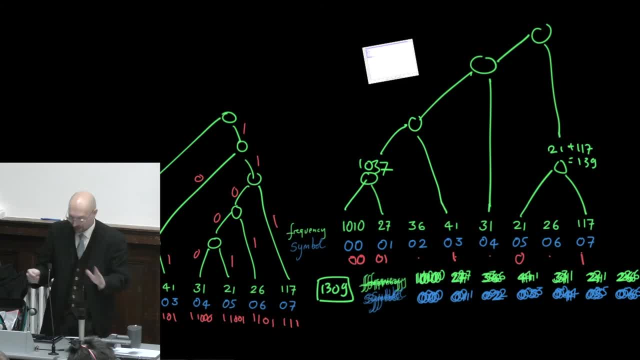 But you are in an elite because other people got lost at some point and are not following anymore. But they will have to work it out. I've made a point of having an exercise in your handout at this stage where, if you haven't been following, you can redo it yourself. 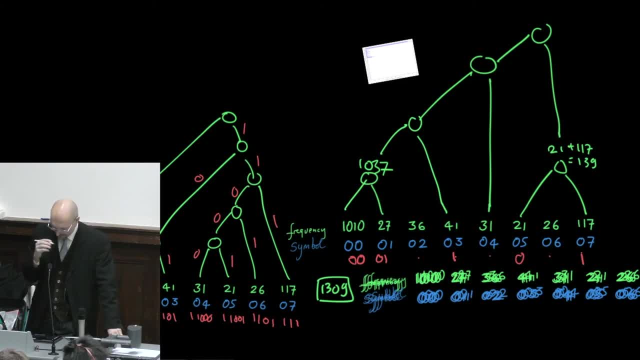 And then hopefully, the coin will click. So at this point I can say: the cost of each decision is the number that I have in here, which is the sum of the frequencies of the things I'm merging and the number that I have in here. 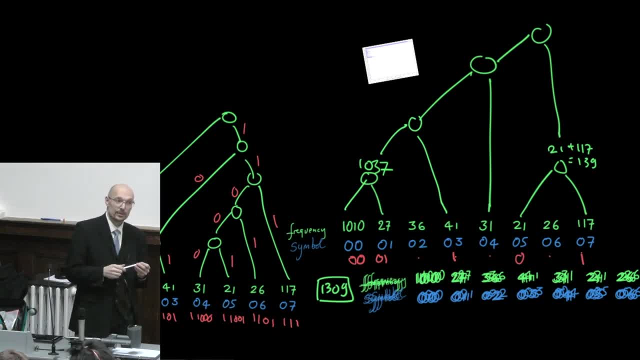 And so the greedy choice would be always to take the merge that has the lowest cost. That's the greedy choice that Huffman takes, And that's how I build a Huffman code. I build a Huffman code by always merging the two lowest frequency emerging things. 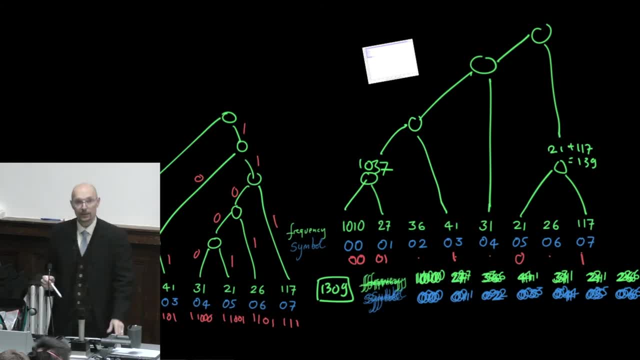 And if I do that I am getting a code that is minimum possible cost among all the abbreviations, And it is possible to prove that non-prefix-free codes cannot do any better And therefore it's worthless even looking at them because they only cause trouble. 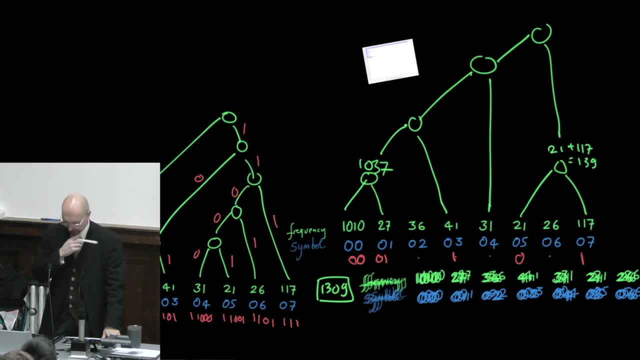 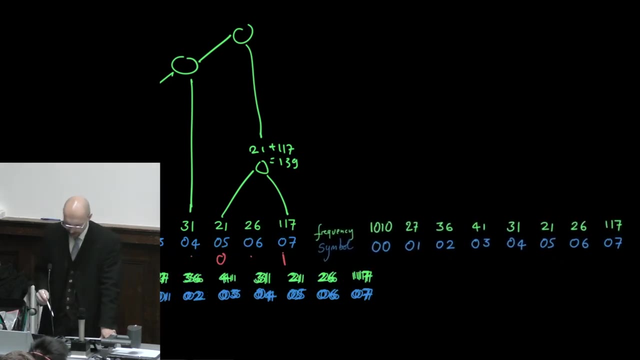 And so it is the best of all these codes, And it's given by Huffman. So what would we do in here? We would start with a blank one. If we wanted to build ourselves a Huffman code, we would build a Huffman code. 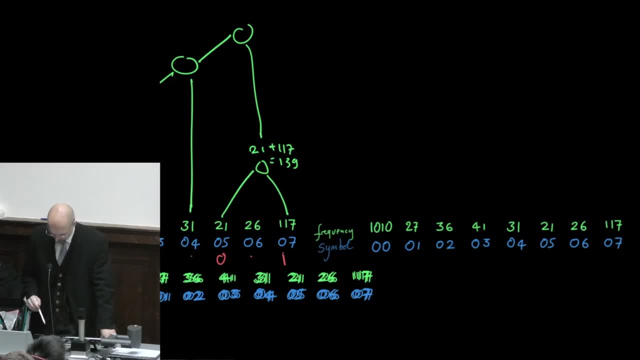 We would take the two lowest frequency symbols, which happen to be 21 and 26. We would make them into a node like this And we would label this with the sum of their frequencies, 47. And then we would take not the smallest two leaves. 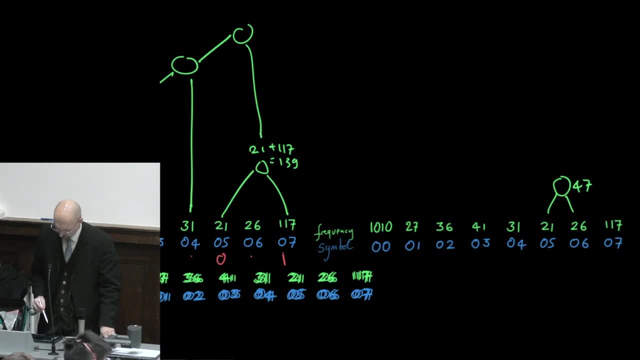 but we would take the smallest two emerging things, So it could be the smallest one. It's this one and this one, which happen to be two leaves, But it could have been a leaf and another tree, and so on. And the way that I actually write the code is to say: 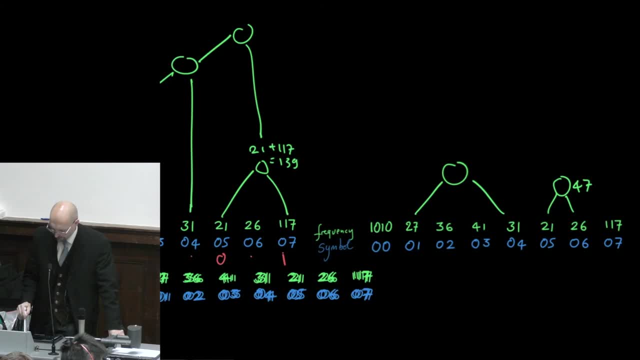 when I build myself this node, which replaces those two with the sum of their frequencies. I also want this to be considered in the sequence of things out of which I will make the next decision. So my easiest thing is just to dump all these frequencies. 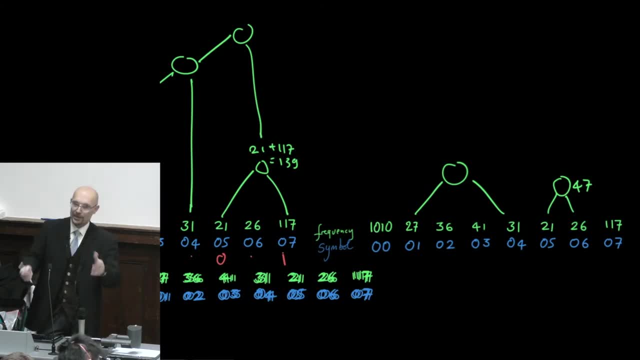 into a min heap and then take the minimum of the min heap twice, add them together and stick it back into the min heap And wherever it comes from, the next two things are going to be the best two things to merge, And I keep going until the min heap runs out of nodes to merge. 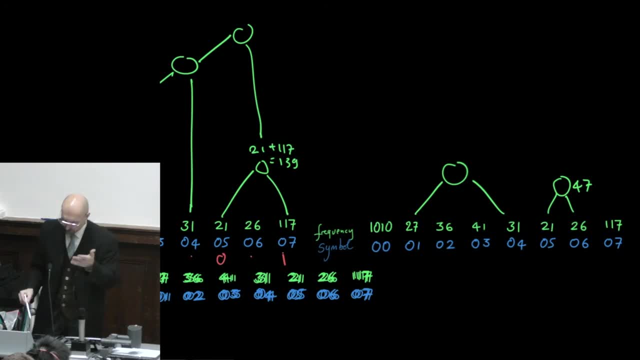 And when there's only one node in the min heap, it means I've reached the root of this tree And then I build the whole code. So this is how you do the Huffman code, And if you were to do that on the example we had, 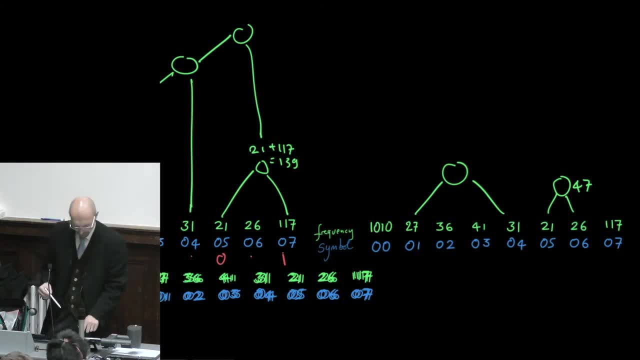 you would reduce things from three bits per codeword to something like 1.58 bits per codeword. I'm not going to try and do it on Blackboard because it takes a long time, But I think I've given you enough. 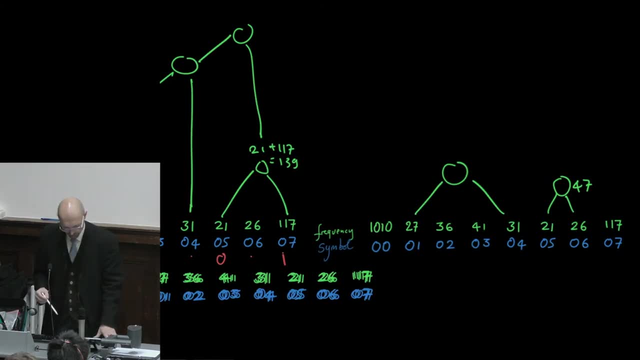 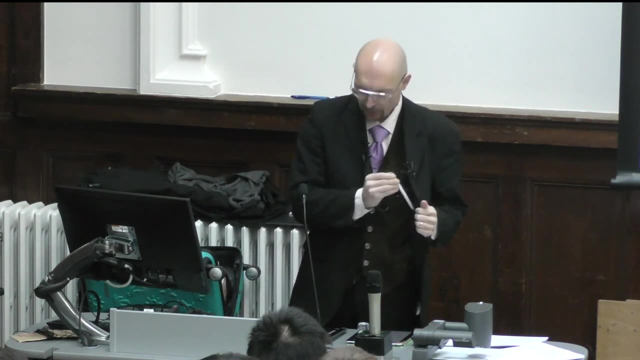 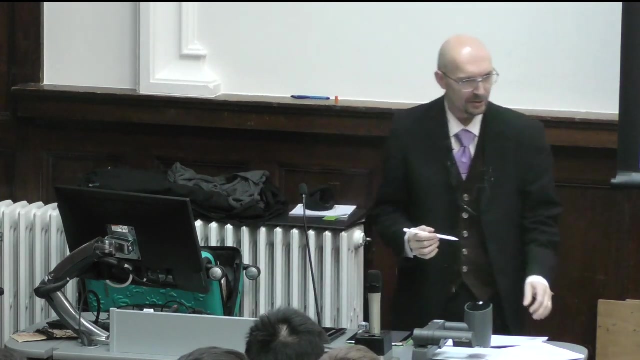 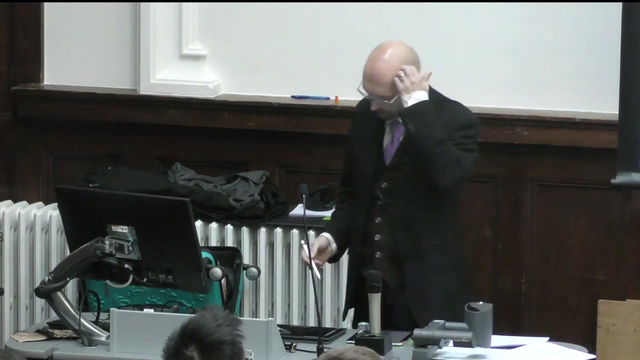 to make you want to go and try it yourself. All right, I am very happy today because I have evidence that some of you have been doing the exercises I suggested in the handout, where there's a blank for you to fill in and do some of these computations. 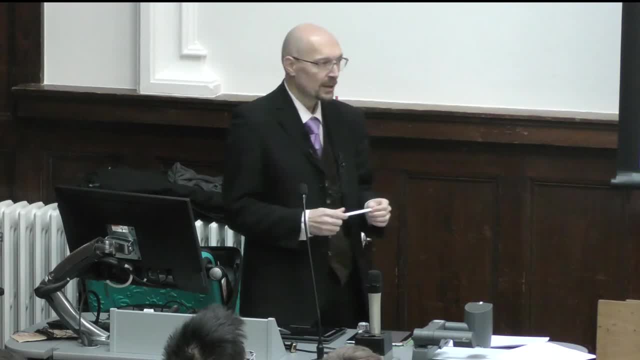 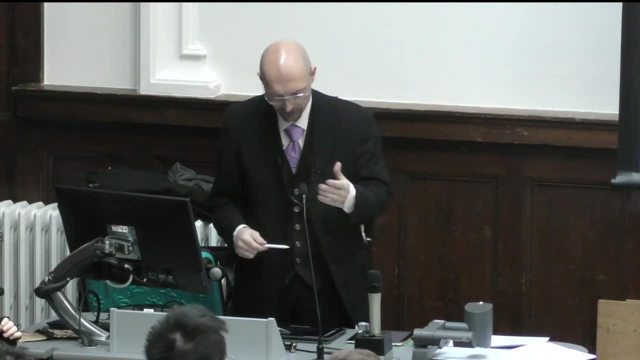 Also, a couple of you came to see me at the end of last lecture And I wanted to ask something that is interesting to share with everyone. I meant to say, but there were so many things to say that I didn't say And I still wanted to say, so I'm going to say it now. 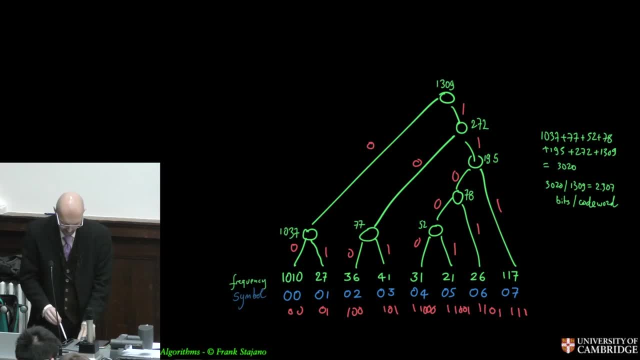 So when you are building up a code- not necessarily the Huffman code, which is the best, the optimal code- you're building a code, any prefix code, out of some symbols for which you know the frequencies. You build the code. You can build it by combining some trees. 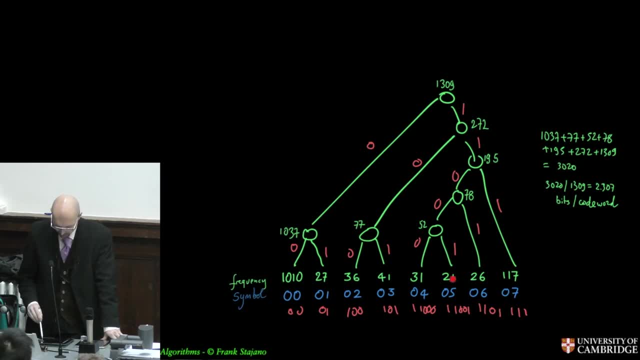 and recording the aggregate frequency of the things you merge. So this one had 31 and 21.. You merge them together, then you add them up and it's 52. If this whole thing had an aggregate frequency, these four symbols together, you added this up, it's 195.. 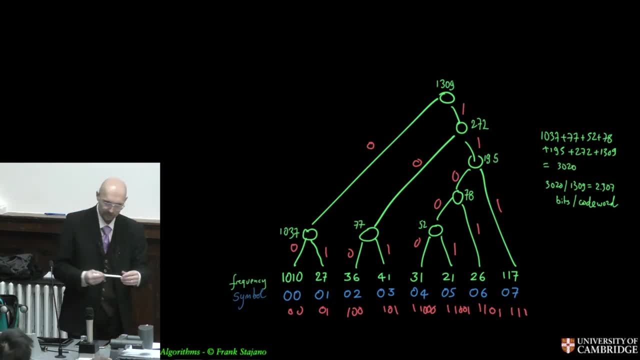 aggregate of over everything is 272. okay, so that's pretty obvious. the thing that is subtle is that the contribution of each decision to the total cost of your code is exactly the value that's in the node of the two things you merge. so every time I decide to merge something, I'm taking a decision because I could. 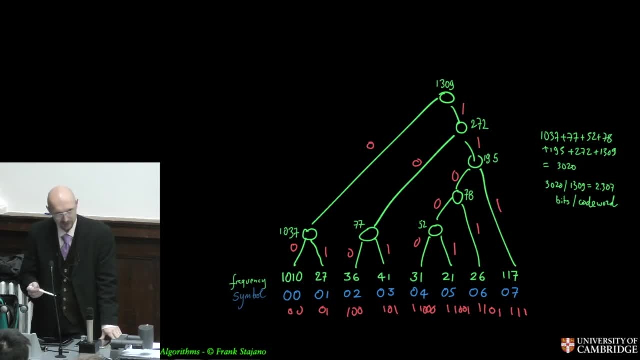 have merged two other things, and the cost of that particular decision is the number in the node. so the sum of the two things that I am merging- and the cool thing is that each one of these is a contribution to the total cost- if you add all of these together, you get the total cost of the code. so you can then. 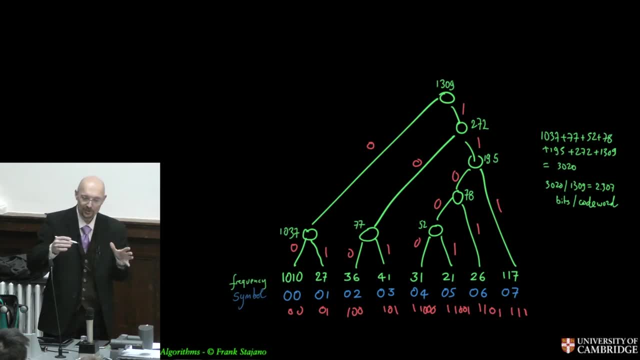 go back and say, oh yes, the code costs a lot because, principally of this decision I made, and if you started by merging this and this, for example, 10, 10 and 27 makes a thousand and 37- this is because at the time you only have these, at the time, the 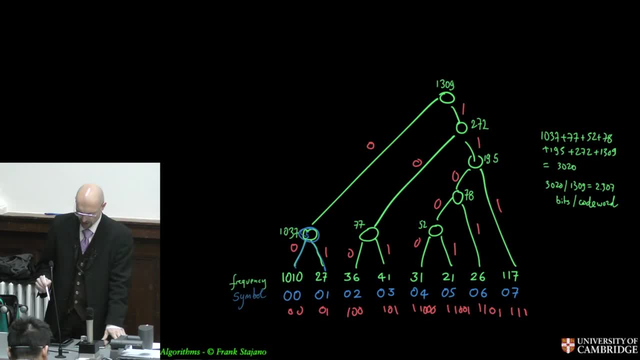 only decision you've taken is this: then you have a forest whose cost is having one symbol, and of length one that would be just zero for this symbol, one symbol of length one to this one, and this symbol occurs a thousand and ten times. this symbol occurs ten, seven times. each of them has length one. so that's the total cost when. 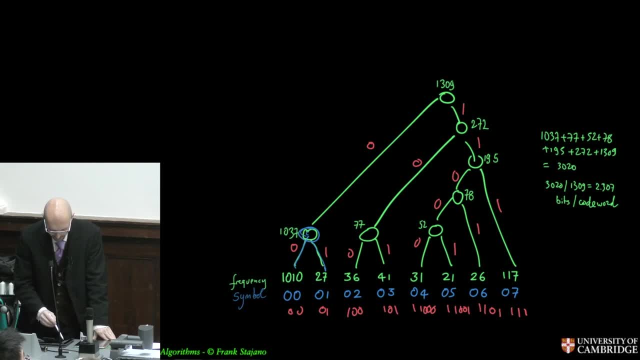 you had another one in, for example, this one. then again you've created two more strings of length. one one- this one over here- occurs 31 times. this one here occurs 21 times. so you add 31 and 21 to the cost, and this is not yet the code, because there are things that are two different symbols. 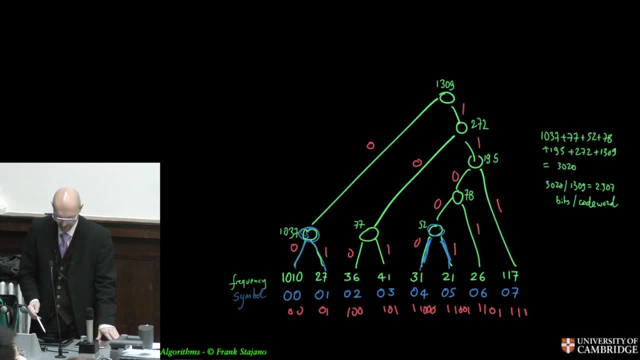 that use the code word zero and a number of symbols that don't have any code words. so it's not a proper code, but this is its cost. so far now, the total cost of my code is the sum of these numbers in here, each one of these blobs together and each one of them incrementally at the time.